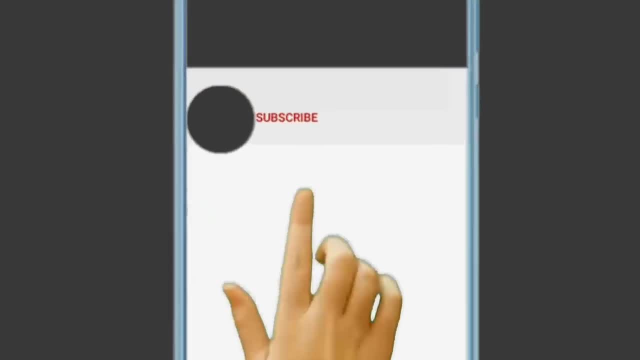 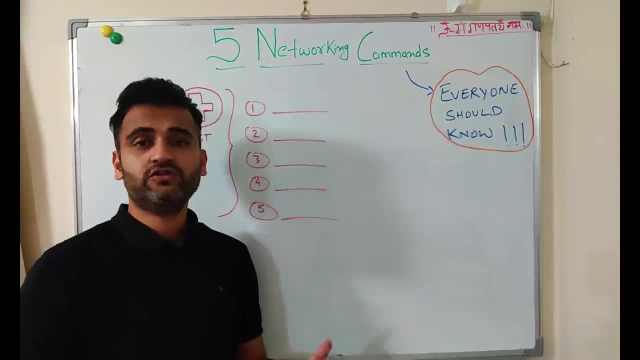 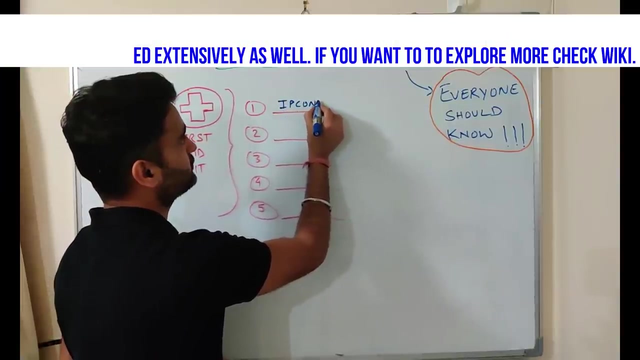 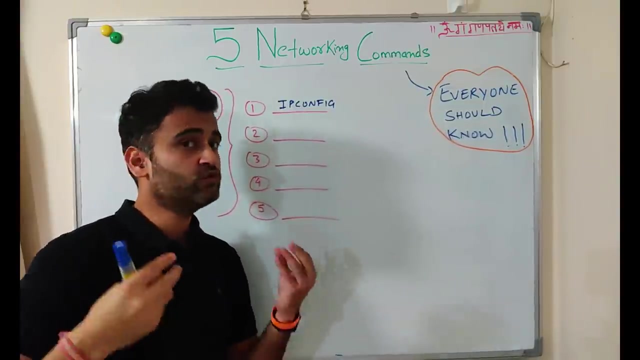 in future. So let's get started. So the most basic command- I think you have already used it a lot- is IP config. I know you already use it, most of you already know, but again, this is for some who does not know a word about networking. 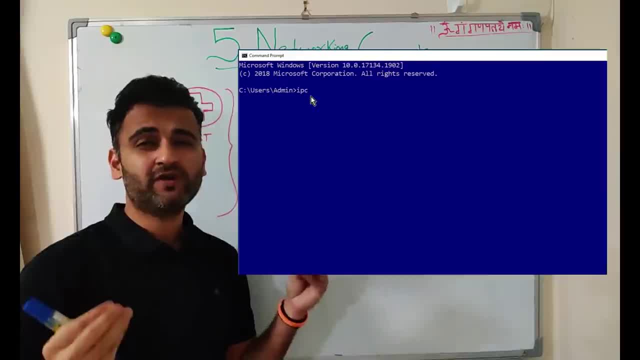 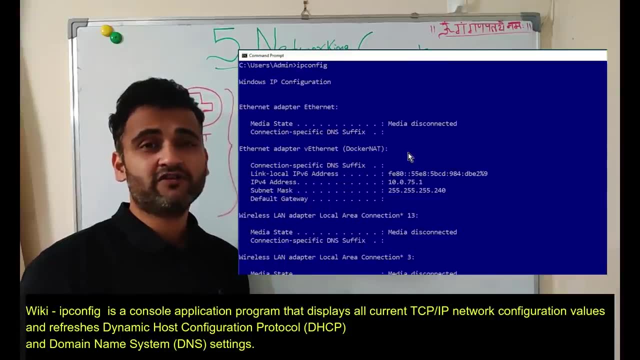 So IP config gives you the bio data of your network. It will give you all the details which are required to exactly understand what is your IP address, what is your DNS, what is your gateway, all those kind of information. and there is a special switch if you use IP config. 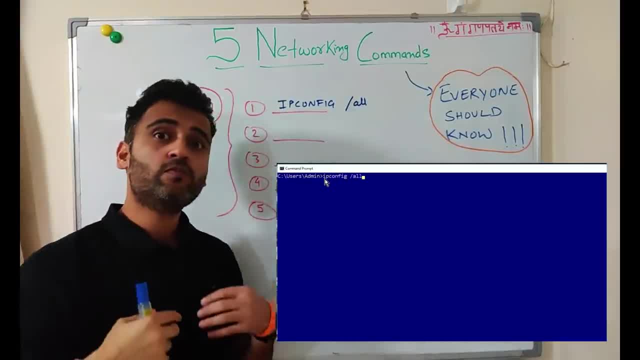 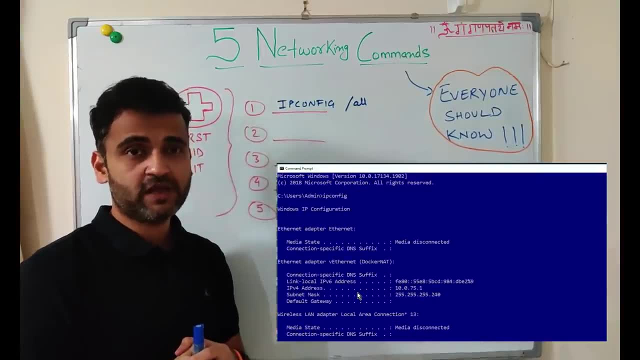 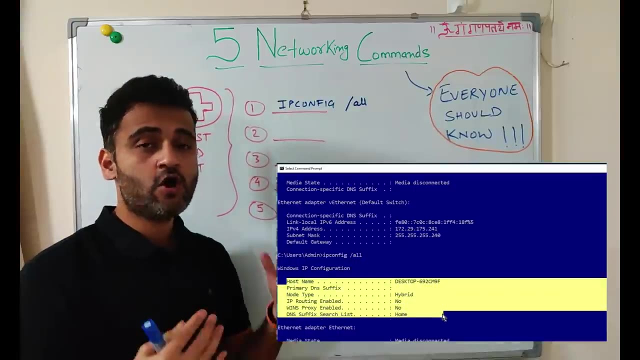 with a slash all switch, then it will give you much more information than a standard IP config command. It will also give you the host name of your particular machine, and this will definitely help you understand that. okay, what exactly the network configurations are there on your machine? 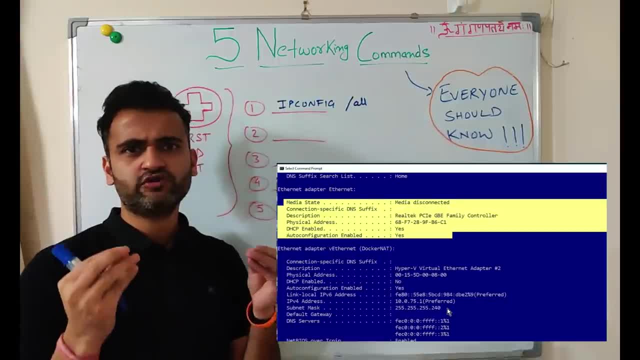 So whenever you are finding any kind of networking issues, you should first try to understand what is your network configuration and what is your IP address, what is your gateway, all those kind of information. and there is a special switch if you use IP config with a slash all switch. 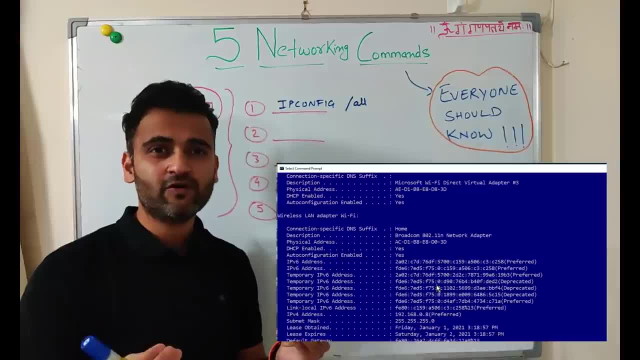 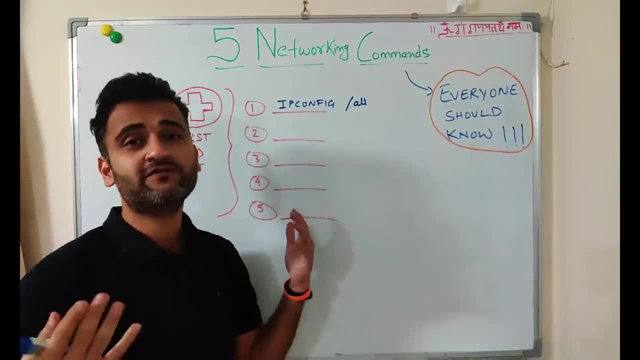 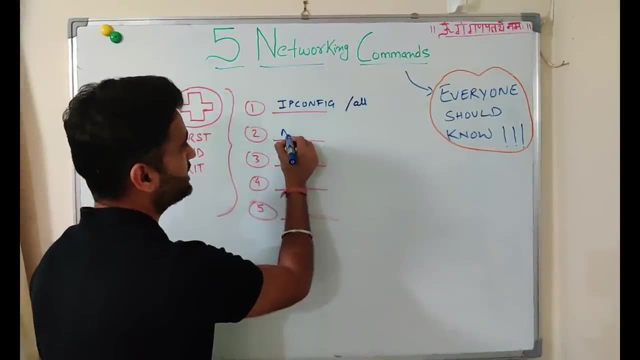 to understand the IP address, the subnet mask, the default gateway, all these kind of information. So suppose, if a network administrator comes to you, you should have all these information ready, which will help you save time. The second command is NSLOOKUP. NSLOOKUP is the command. 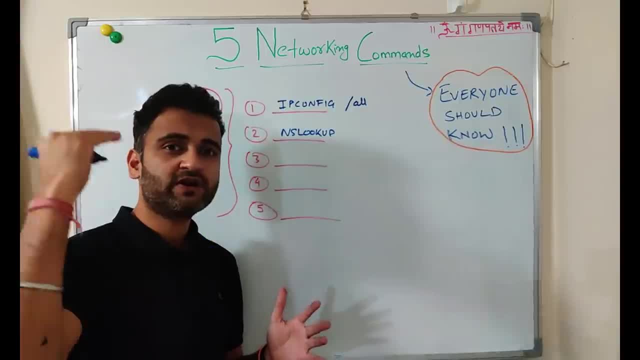 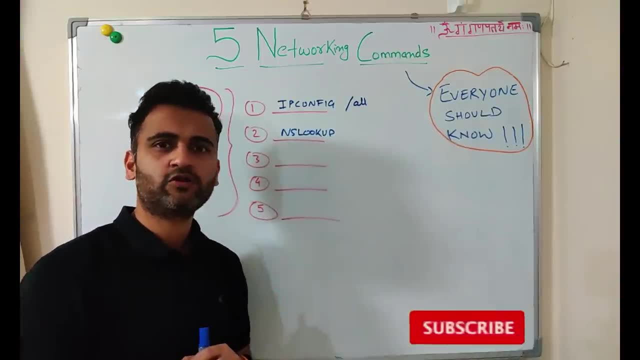 which exactly, if you follow it it will give you that. okay, which particular domain name server will be supplying you the IP addresses of any particular, you know any particular domain name which you are trying to query. Suppose, if you are typing wwwgooglecom, then from where exactly the IP address would be coming for that particular? 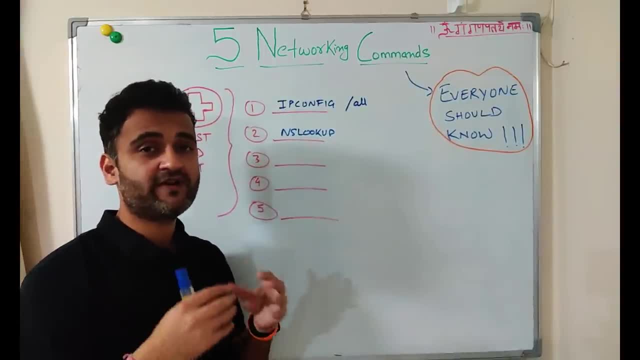 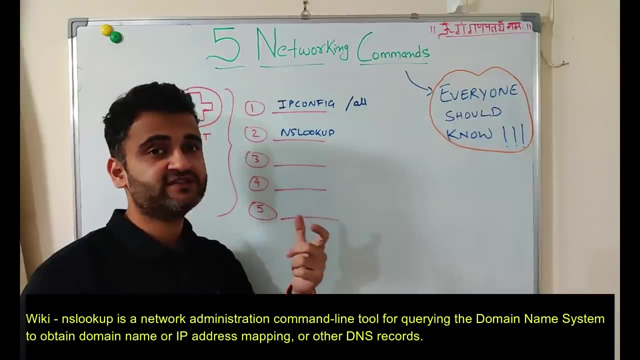 domain name. So this is what will be given by your NSLOOKUP. When you type the NSLOOKUP, it will give you the domain name server IP address where you know you can identify that, okay, this is my name server. and then it will. also, if you add, you know the domain name which you are looking for. 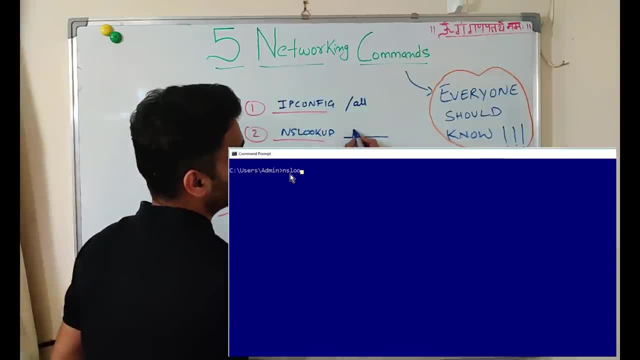 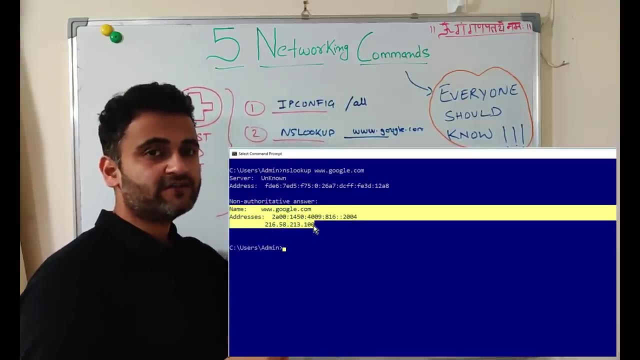 So suppose you have a website, wwwgooglecom, So suppose if you are doing a NSLOOKUP on that, so it will give you the DNS server from which this particular query will be queried and also the IP address of the underlying server, which you know. 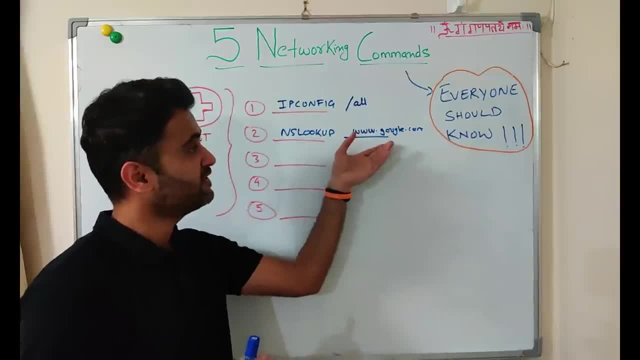 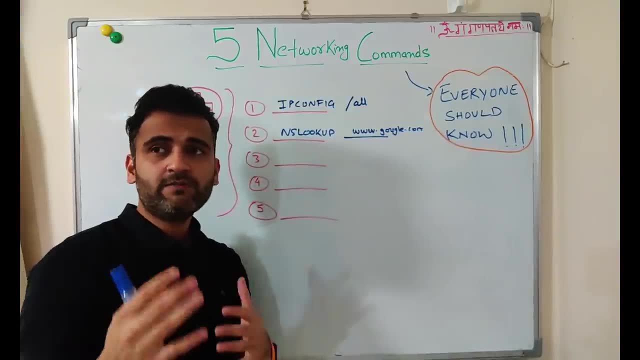 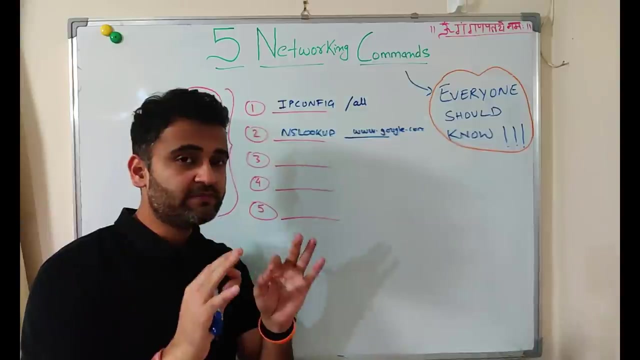 which you are trying to query, So in this case, the IP address which will be resolving to your Google server Now, where it can be used. Suppose there is a scenario where you are able to reach one of your application using its IP address- okay, but when you are trying to type the host name of that particular application, it is not reaching. 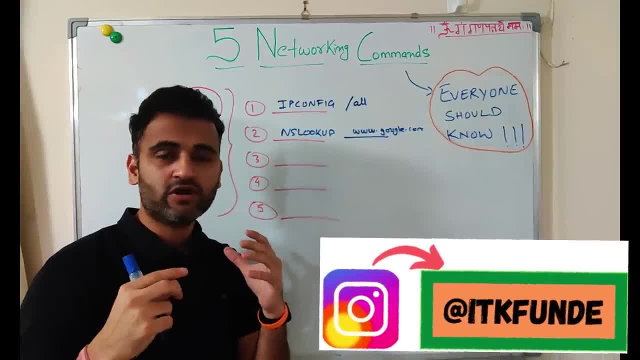 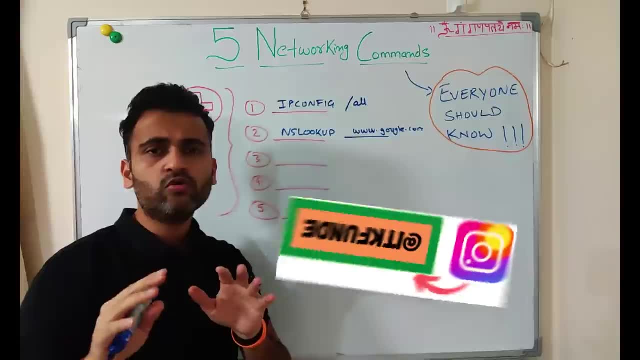 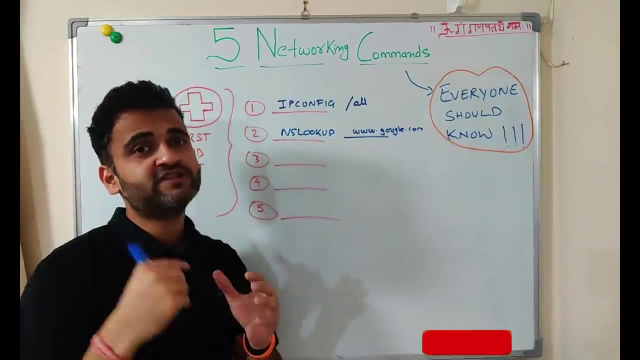 and you are getting some error that you know: not able to recognize the name or something like that. some error, some random error you are getting while you are typing the host name or the domain name of that particular application. Now there can be a reason of you know some issue with the DNS, so what you can do is a domain name server can also do a. 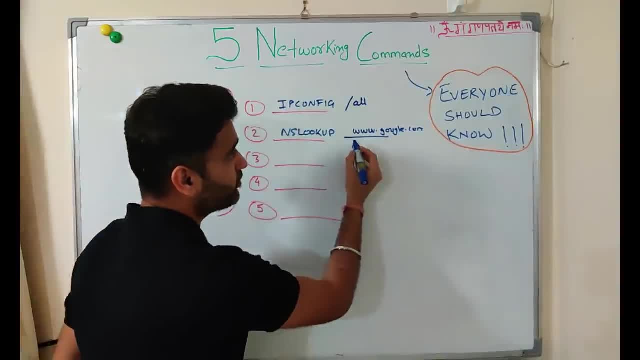 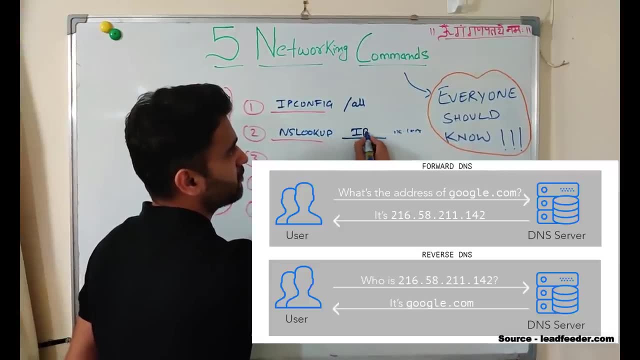 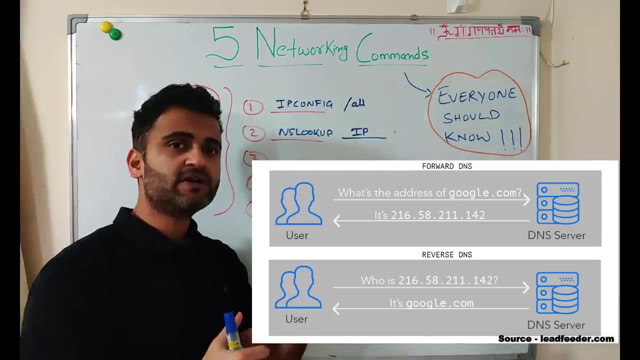 reverse lookup. What is the reverse lookup? that, instead of passing the domain name, if you pass the IP. okay, if you pass the IP, then it will tell you that, okay, this is the particular domain name it is resolving to. Okay, so it might happen that. 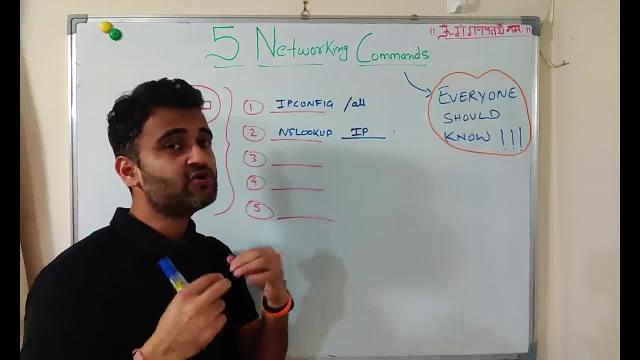 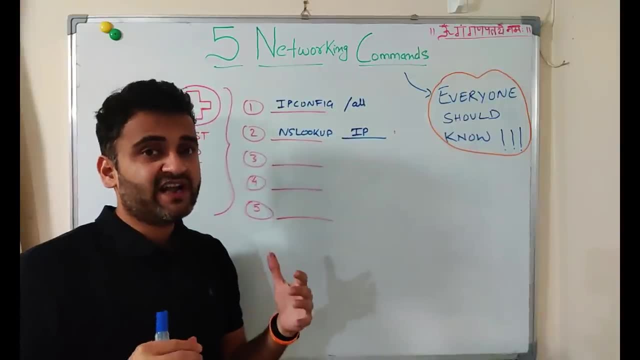 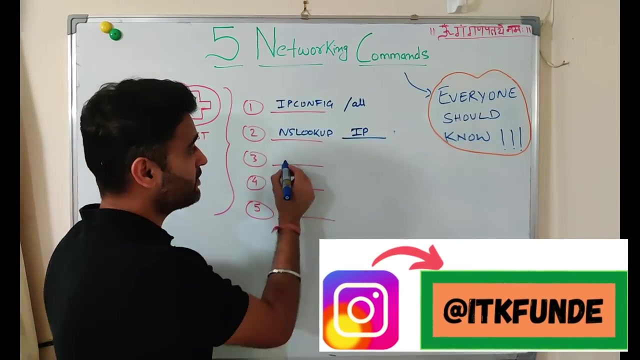 the IP which you know, which you are trying to reach, is not exactly assigned to that particular application. so NS lookup is a very good command if you are trying to identify and fix DNS related issues. okay, so this is an NS lookup, a very useful command. another very basic command is the ping command. ping is 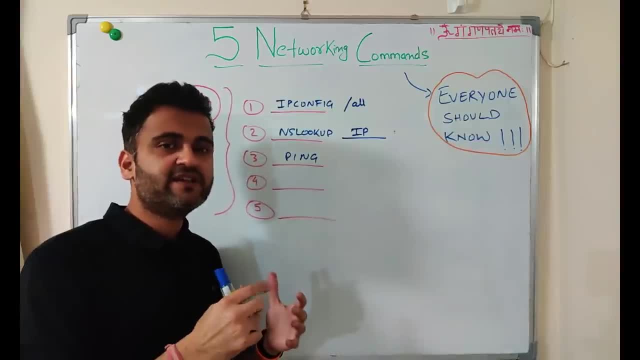 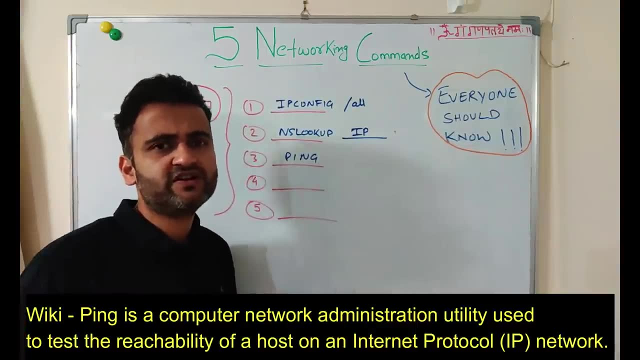 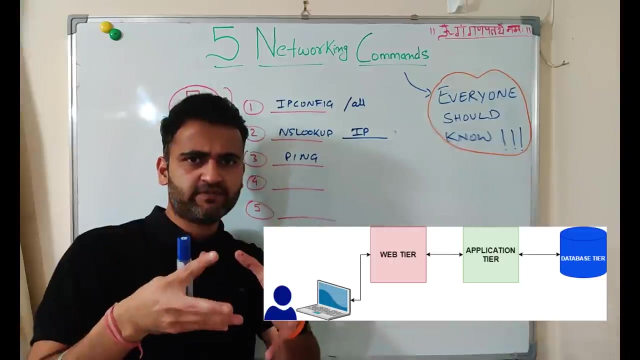 simply a command wherein you try to understand whether a particular host is reachable over the network or not. so suppose, if you want to test, suppose your application is not working okay and your application is. you know, your application is a three-tier application. where there is a web server, then there is an. 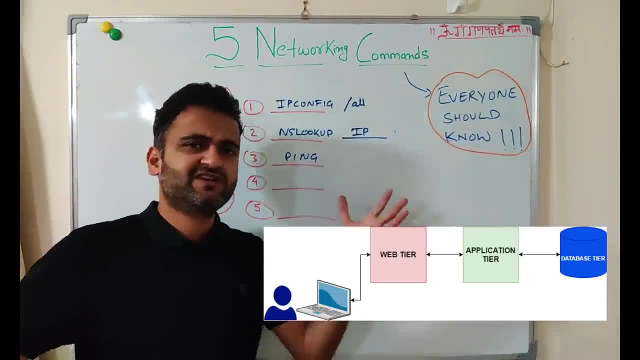 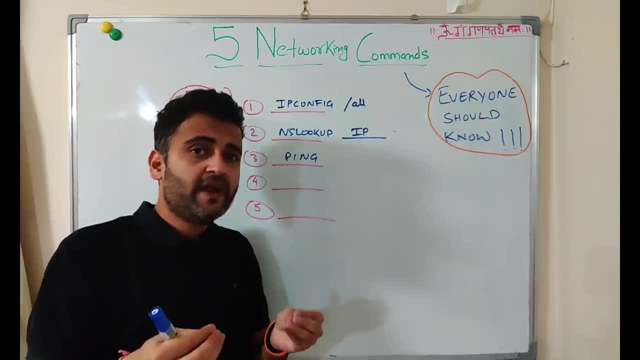 application server and then there is a database database server. so it's a three-tier architecture and whenever you are hitting you are getting some error. so the basic thing which you can do is you try to ping the first server with which you are making that connection. okay, try to ping that server. 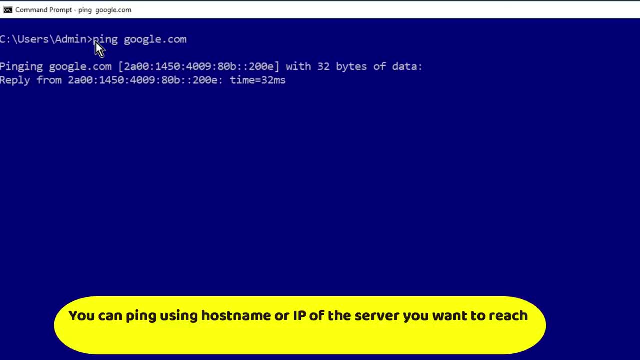 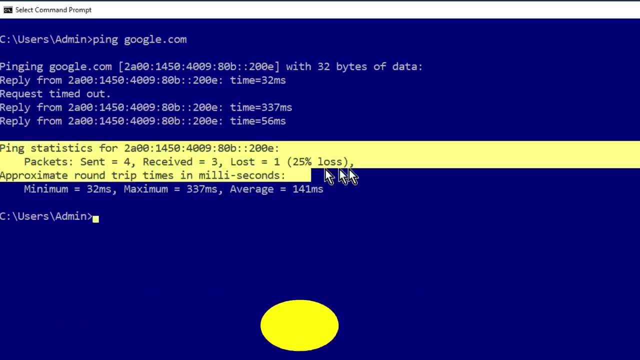 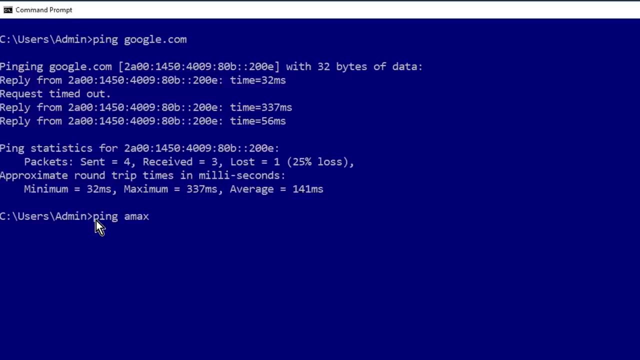 simply see if it is reachable or not. suppose you are trying to hit you know some query on the database server but you are not able to establish the connection. try to hit that particular database server with this ping command and understand that, whether the response is coming back or not. okay, so ping is again a very, very 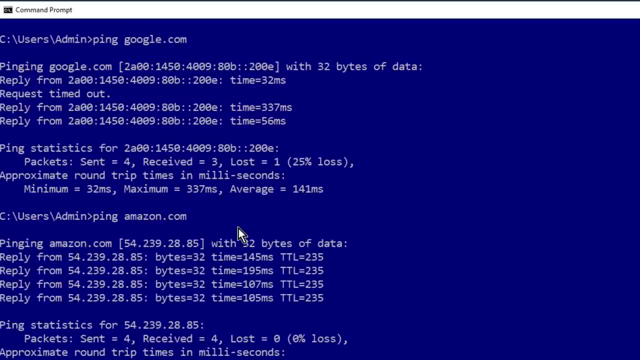 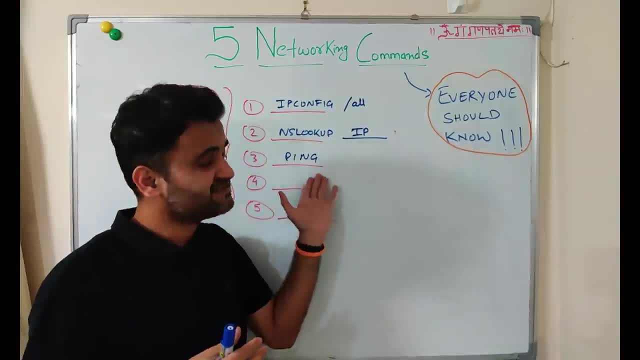 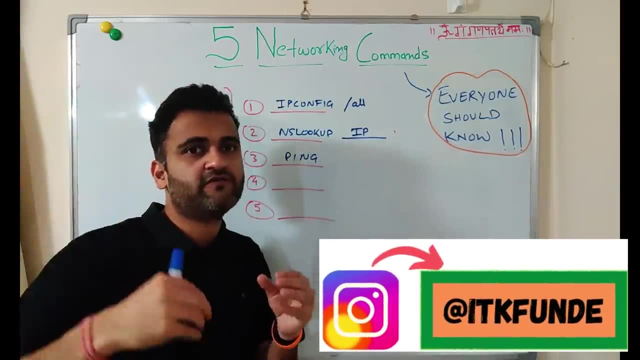 important command, and all these commands have very, very advanced switches which can further enhance the capabilities of these basic commands. so for that you have to use the documentation, but just remember that is also, you know, an evergreen command whenever you try to check the reachability of any particular. 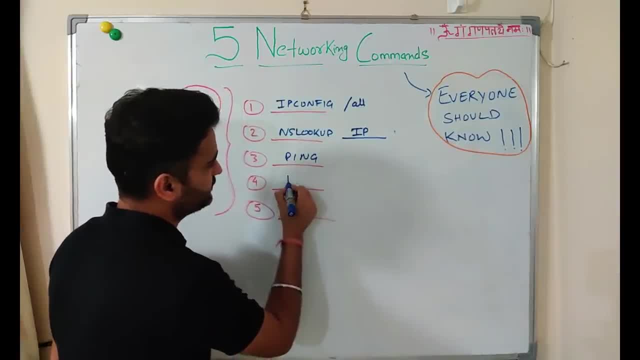 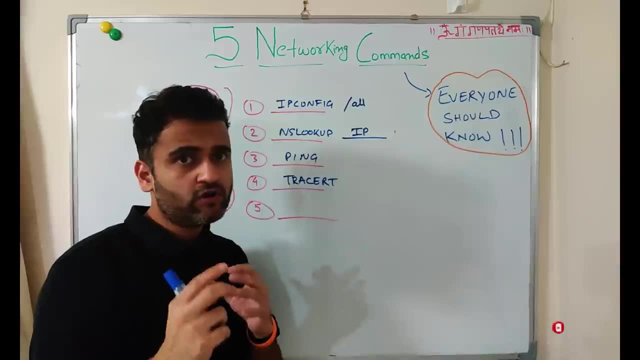 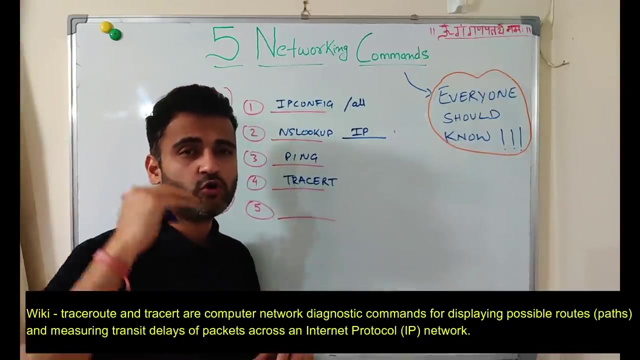 server or service. The next command is traceroute. Traceroute is a very, very good command if you are trying to diagnose some sort of a performance issue, because traceroute, as the name suggests, when you do a traceroute on to a particular destination, this particular traceroute command will show you all the hops. 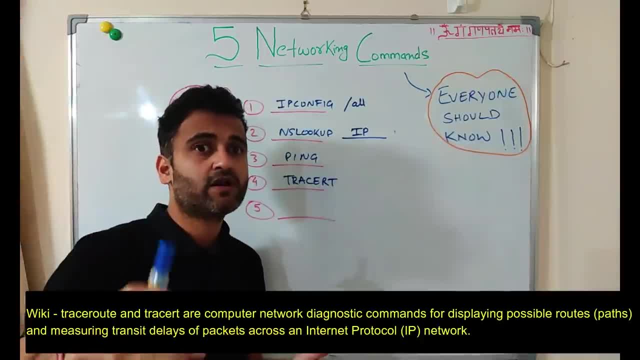 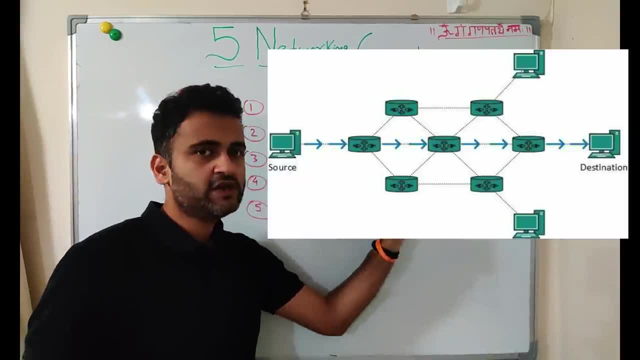 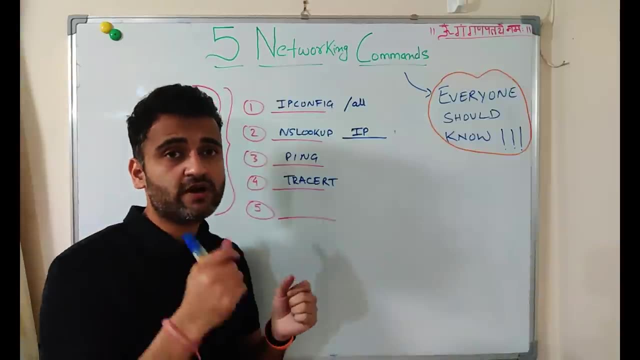 which, particular, with that particular packet, takes over multiple routers. So suppose you are a source and there is a destination you are trying to connect to the destination. so there must be, you know, different network devices with which the packet is going to that particular destination. So this particular traceroute command exactly tells you whether you are able to go through. 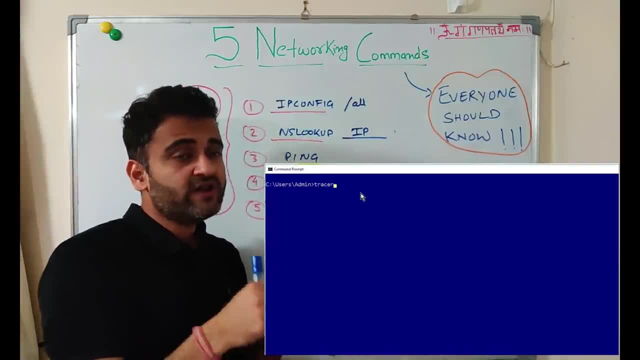 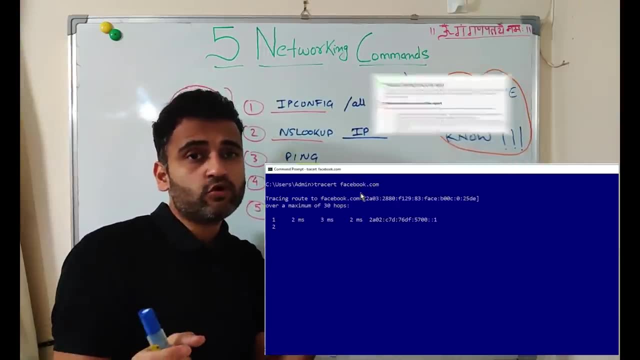 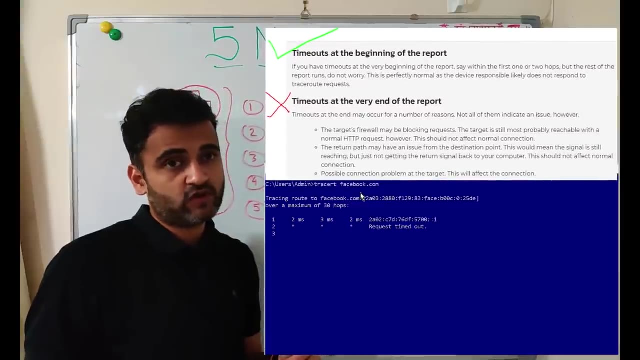 those hops correctly or not? And suppose When you are doing that traceroute you are seeing that in one particular hop the request timeout is coming. request timeout means that at that particular hop that particular router is not further passing the packet to the next router. 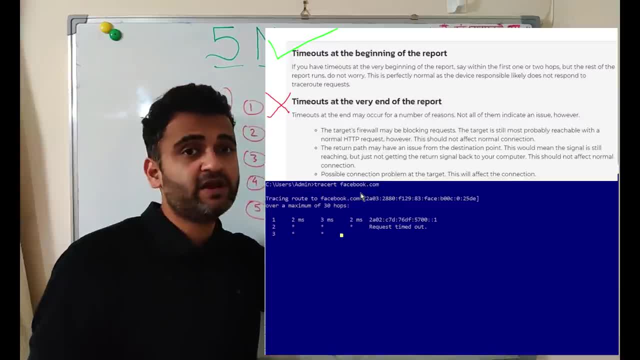 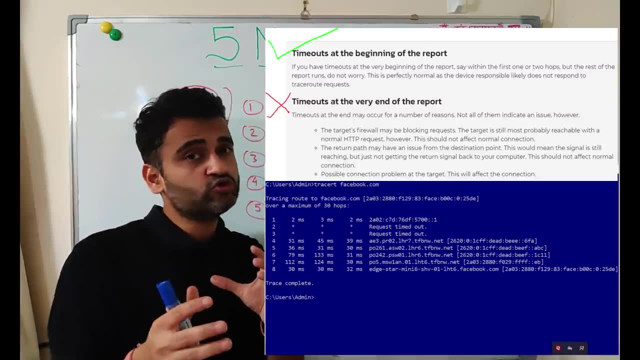 So always look for those signals. and also it also give you the time it took for sending a packet from one destination, from one source to the destination. So that also goes to show that okay, in one particular hop, whether it is taking more time than usual. 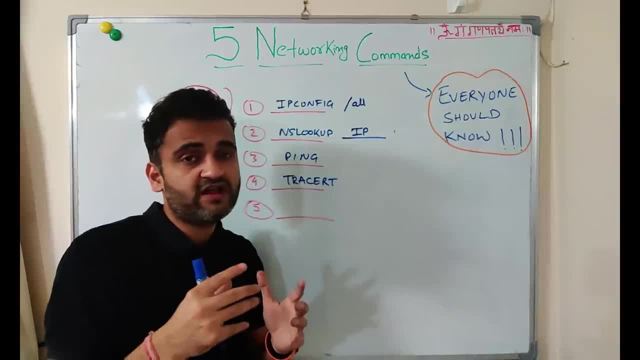 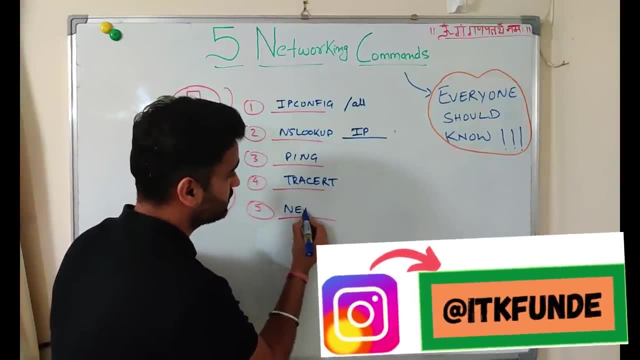 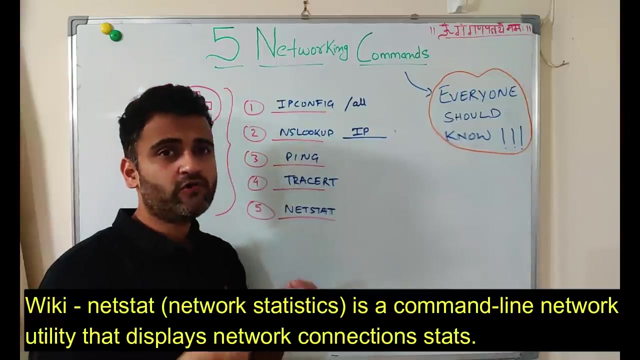 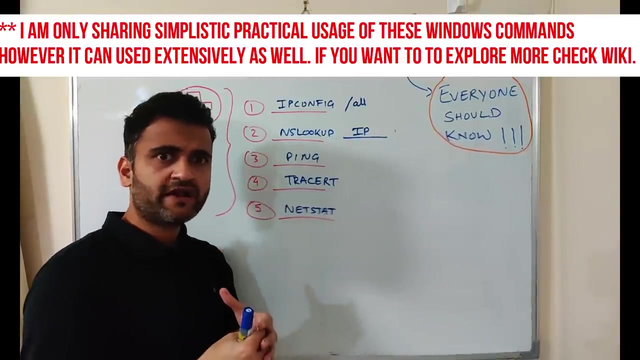 So traceroute, again a very important command when you are trying to identify intermittent performance kind of issues. and the last command is netstat. Now, netstat command is used to identify all the active connections you have over over the network. Okay, so whenever you try to establish any kind of TCP IP connections, you know you connect. 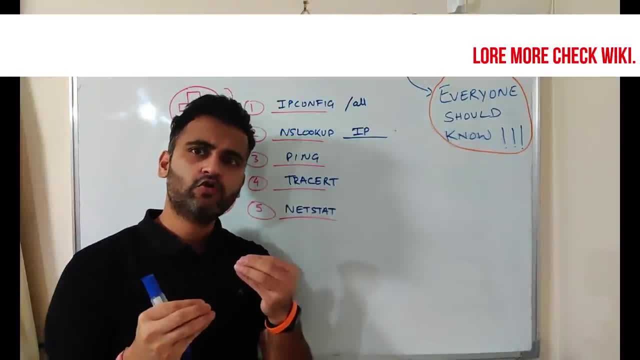 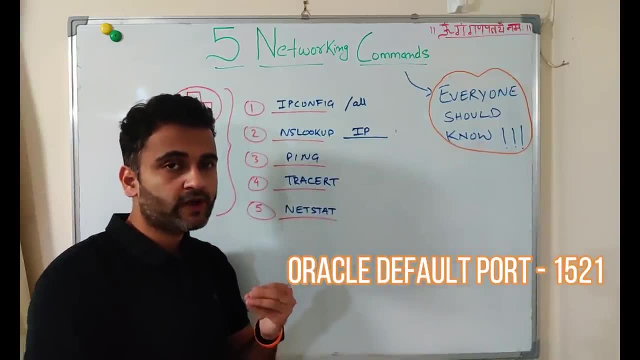 to a particular port. suppose, for example, you try to connect to an Oracle database. Now, what is the default port for Oracle database? people who don't know, it is 1521, okay, So you have to see that, okay, whenever you are doing a netstat, and mainly there is you. 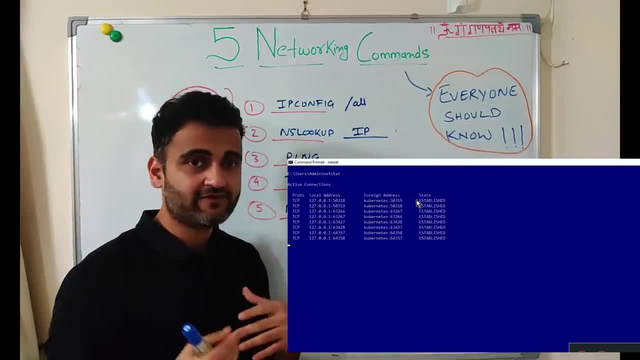 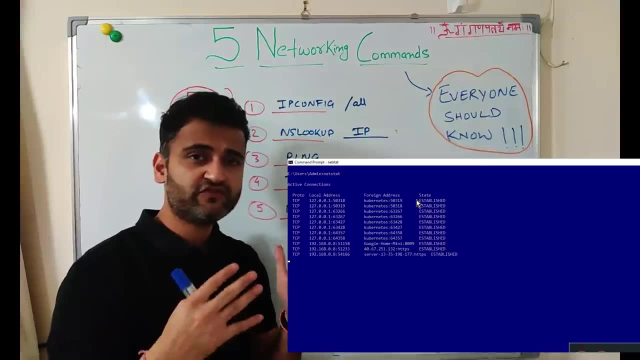 know there is a switch called like an A switch, netstat-A, where in, if you run that, you will get all the list of active connections which are there, which are, you know, which your computer is listening to and the ports of the same. so suppose you are trying to reach a particular? 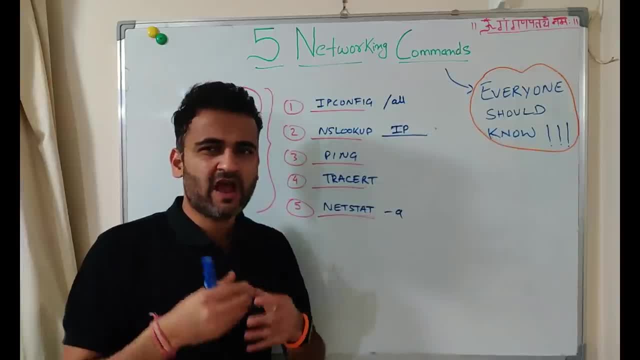 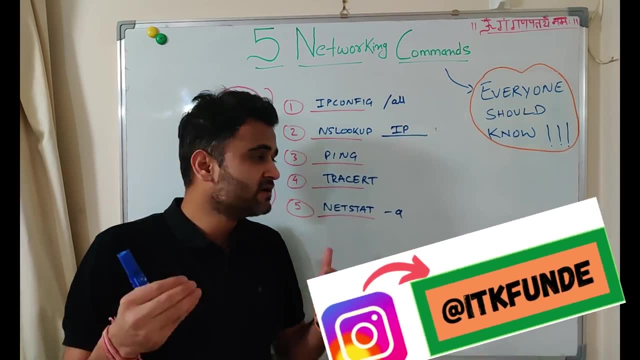 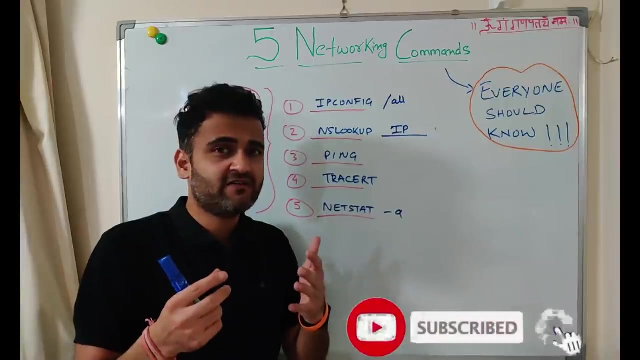 server. You are running over the network on a specific port and you are you are getting error like connection refused or something like that. So in that case it would be worth running a netstat command to identify all the open active TCP IP connections and identify whether there is, you know, this particular port is. 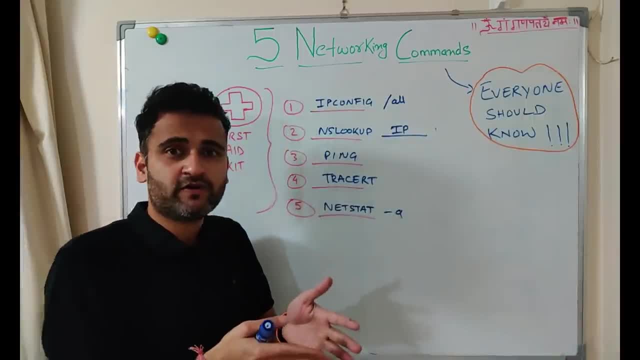 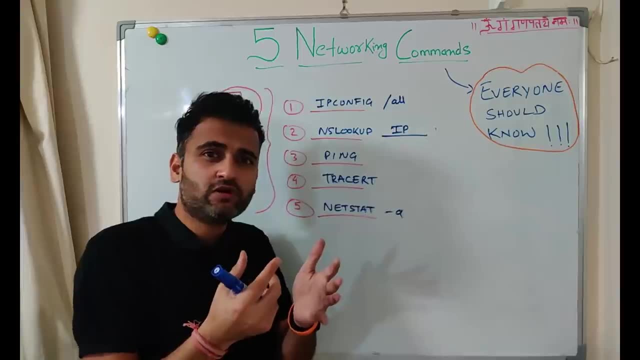 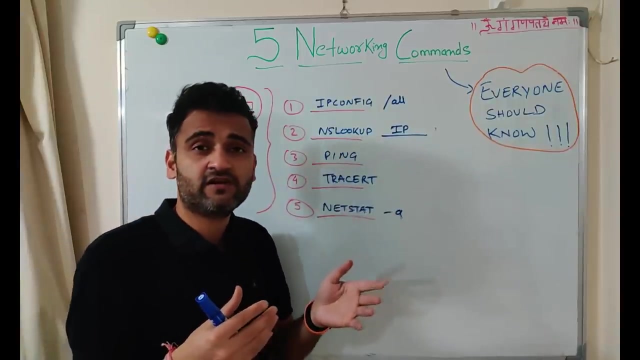 already consumed by by, you know, by some other kind of connection. So this netstat command is very helpful when you are trying to troubleshoot something to do with your connectivity and your open TCP IP connections. There are various switches available for all these commands and based on your understanding. 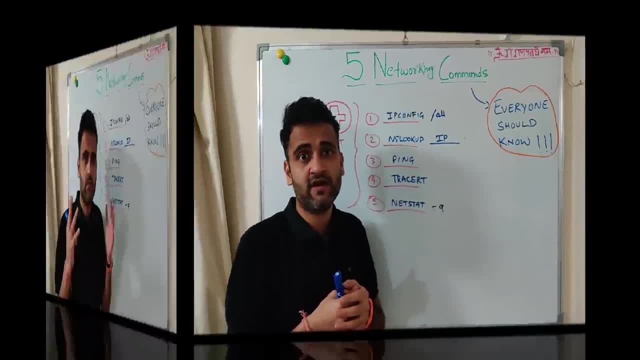 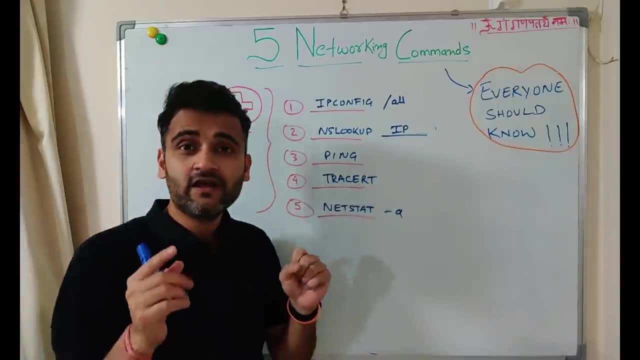 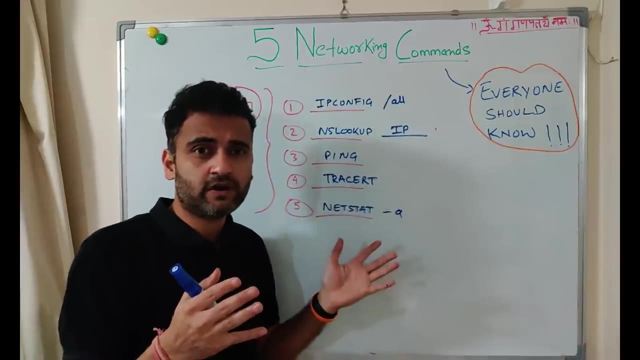 and usage. you can- you know you can- use these five commands. So, friends, I hope you now know what are these five basic commands and how it can form your first aid kit in order to troubleshoot any networking issues. There are a lot of advanced switches which are available to use these. you know, use these. 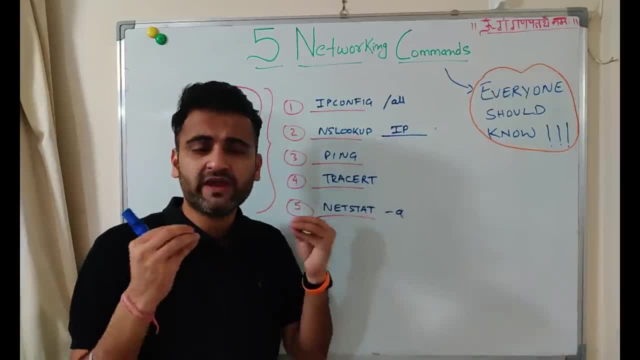 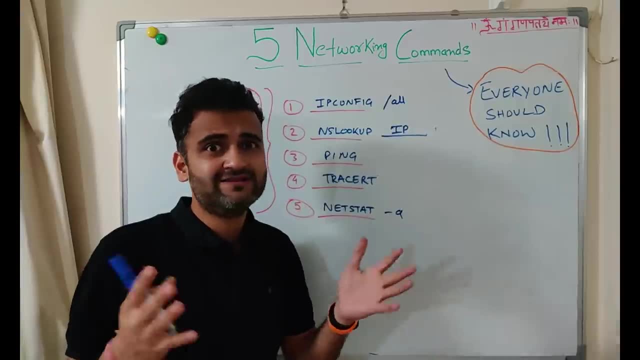 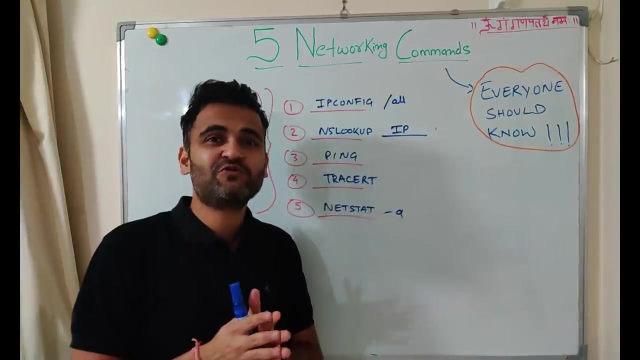 commands. If you are a beginner, I think the basic commands would do in just enough, and once you know something about these issues, you can either contact a network administrator or else you can fix it yourself. So I hope with these five commands you will now have a better chance to look into any 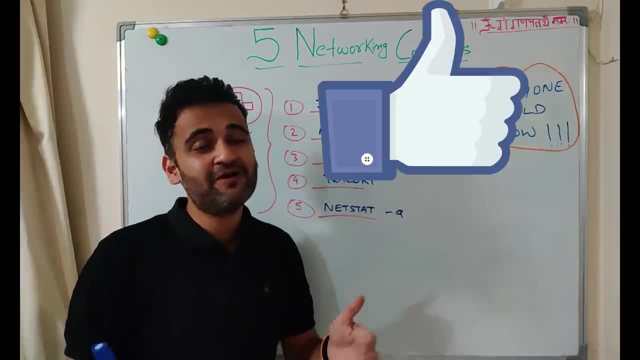 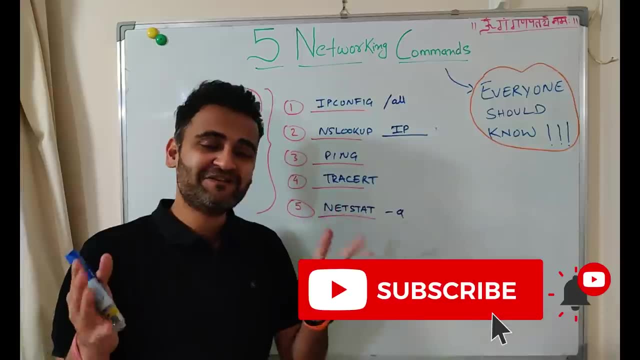 possible network issue. If you like this video, please hit the like button. please hit the subscribe button. if you find this content to be of any use to you, let me know in the comment section what you would want to learn next. we are going ahead with our networking series, but we will. 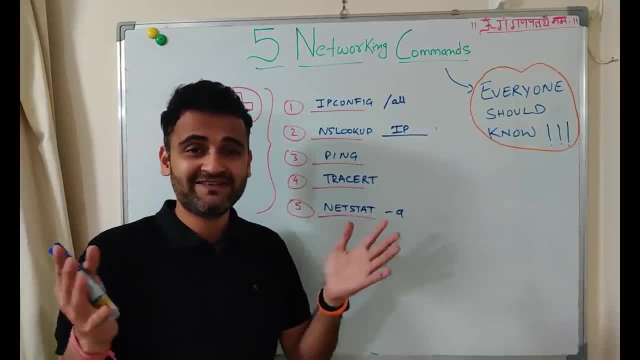 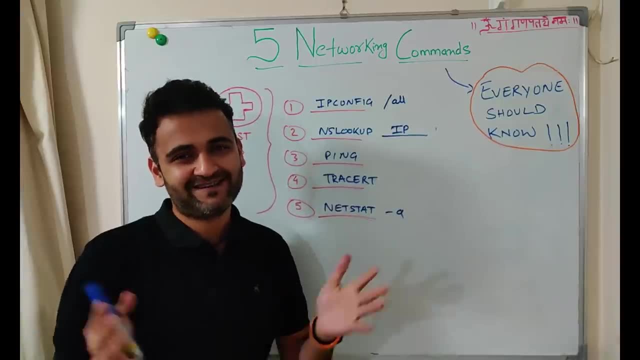 be touching into other areas of information technology. so please let me know and, yes, keep supporting and keep showering all the love on this channel. So until then, keep hustling bye. for now,